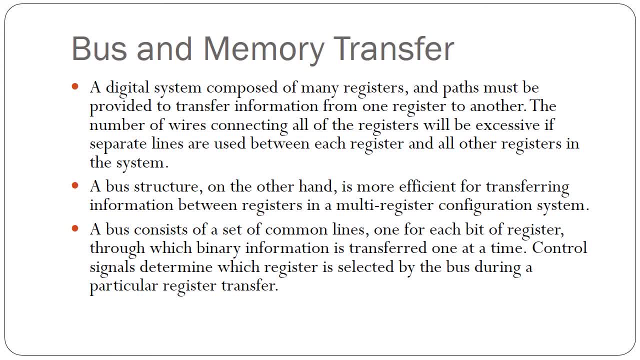 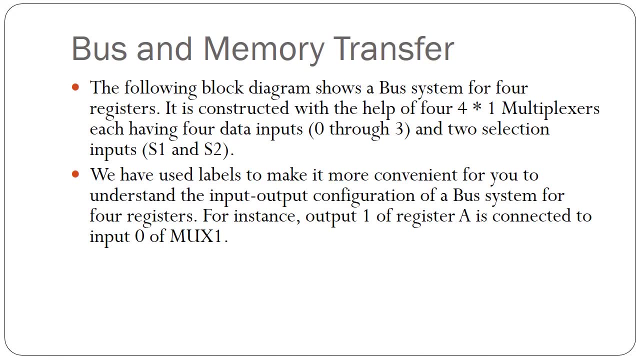 So this is the concept of bus and memory transfer. Here I will show one diagram for bus system, in that there are four registers. It is constructed with help of four into one multiplexer, each having four data inputs, 0 to 3, and two selection inputs. 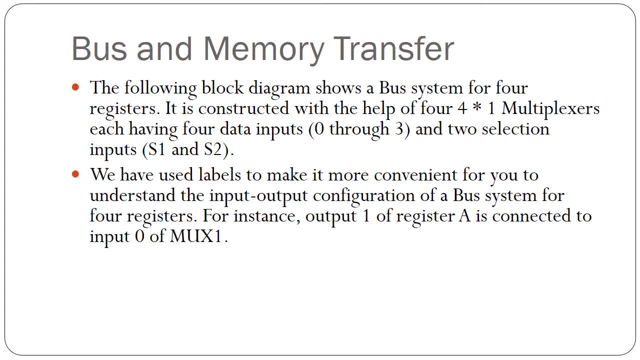 Okay, S1 and S2.. We have used labels to make it more convenient for you to understand the input output configuration of a bus system for four registers. Okay, So here. output of register A is connected to input 0 of multiplexer 1.. 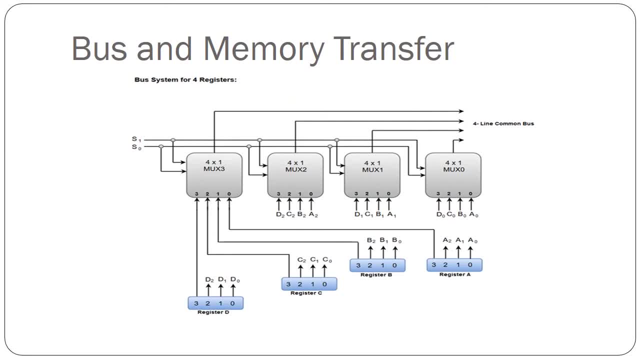 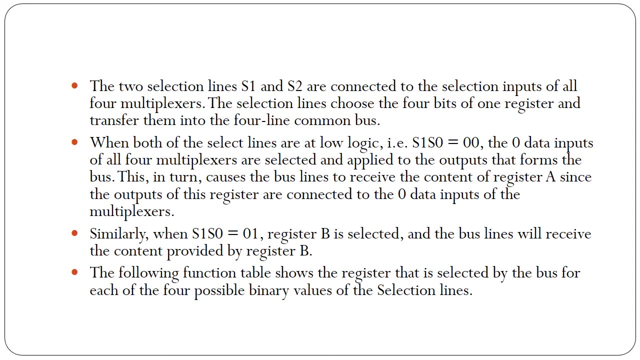 This is the block diagram of bus and memory transfer. Here you can see two selection inputs, S0 and S1.. Four line common bus and there are four registers: register A, register B, register C and register D. The two selection lines, S1 and S2, are connected to the selection inputs of all four multiplexers. 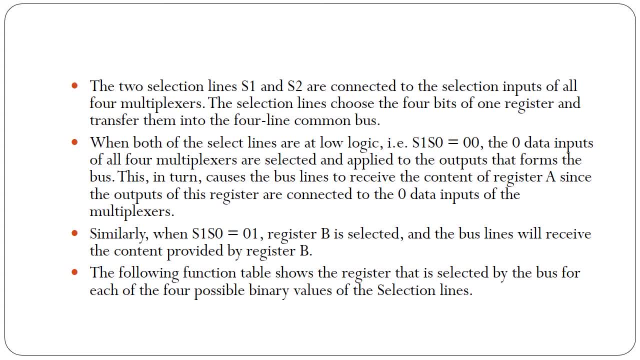 The selection line, choose the four base of one register and transfer them into the four line common bus When both of the select lines are at low logic. suppose S1 and S0 is equal to 0, 0. The zero data inputs of all four multiplexers are selected and applied to the output that forms the bus. 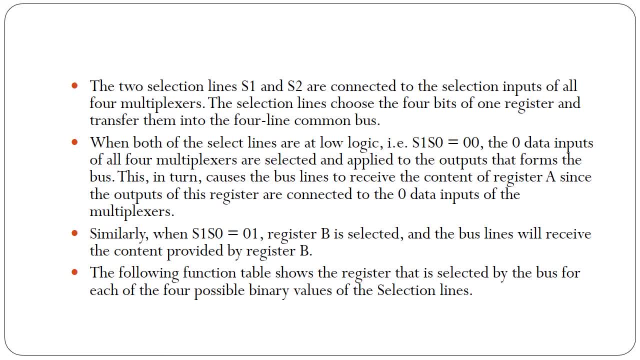 This is, in turn, like causes bus lines to receive the content of register A through the outputs of this register are connected to the zero data inputs of the multiplexer. Similarly, when S1 and S0 is equal to 1.. 0,, 1,, register B is selected and the bus lines will receive the content provided by register B. 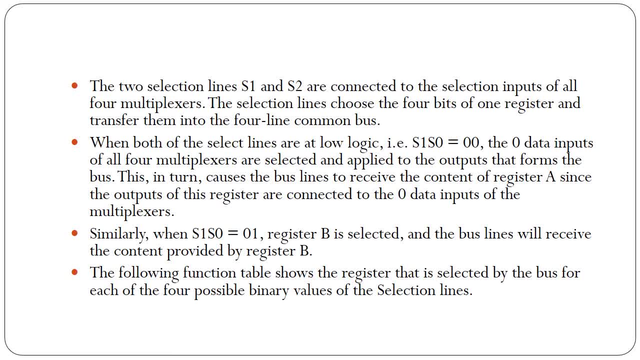 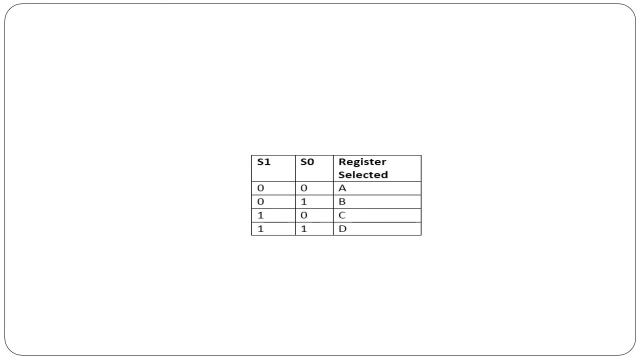 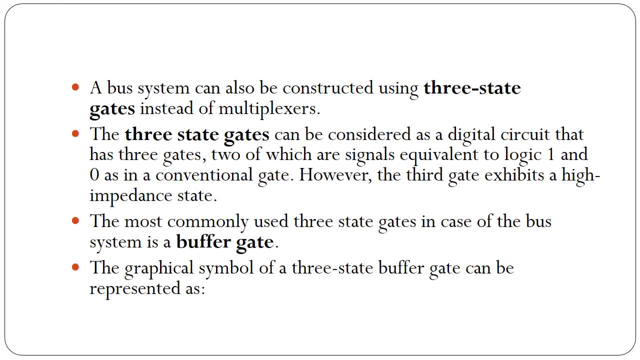 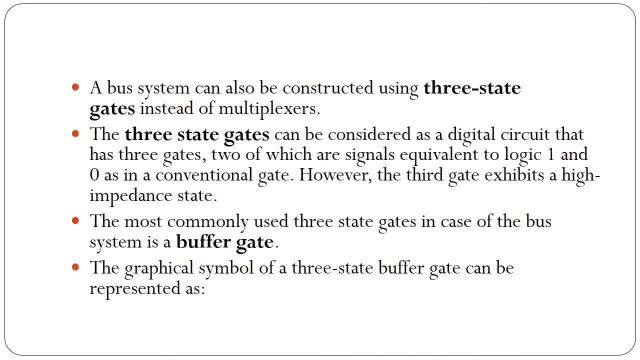 But the third gate exhibits a high impedance state. The most commonly used three-state gate in case of the bus system is a buffer gate. The most commonly used three-state gate in case of the bus system is a buffer gate. I will show the graphical symbol of buffer state in my next slide. 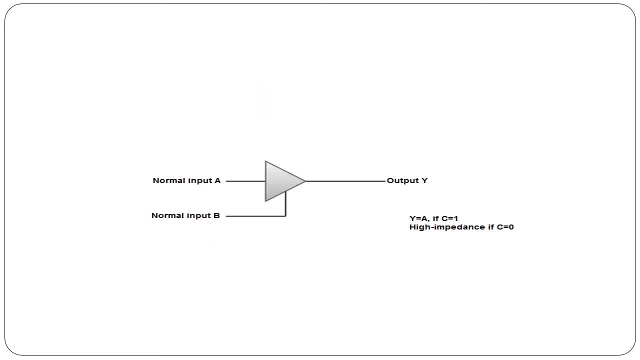 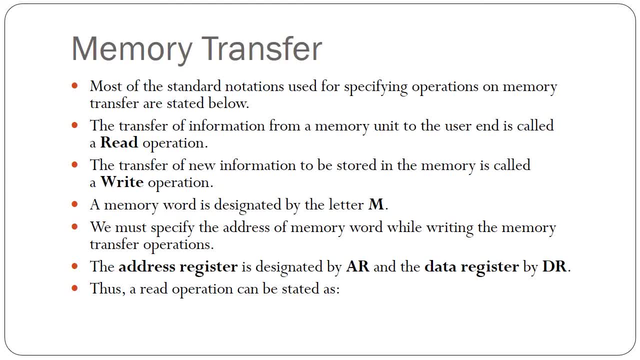 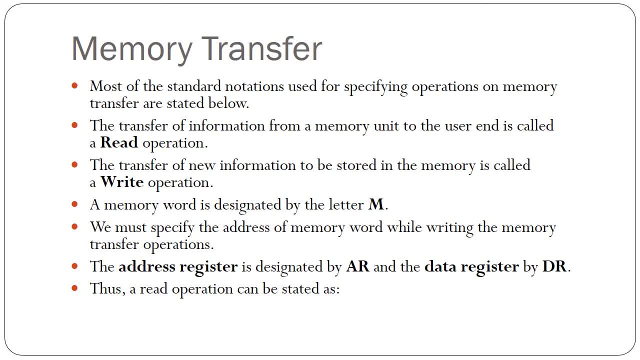 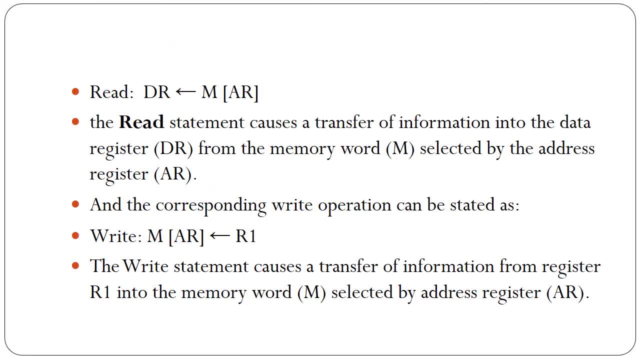 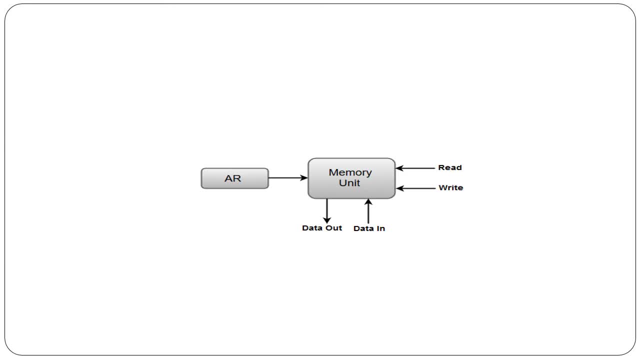 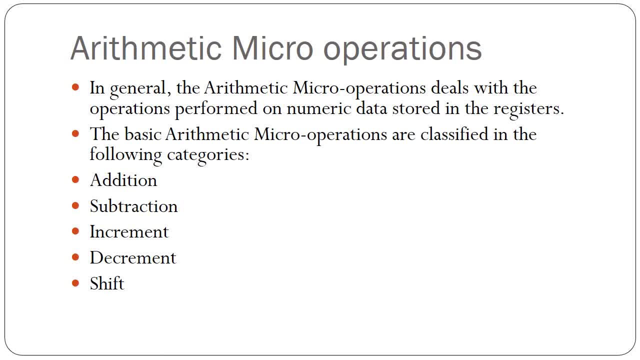 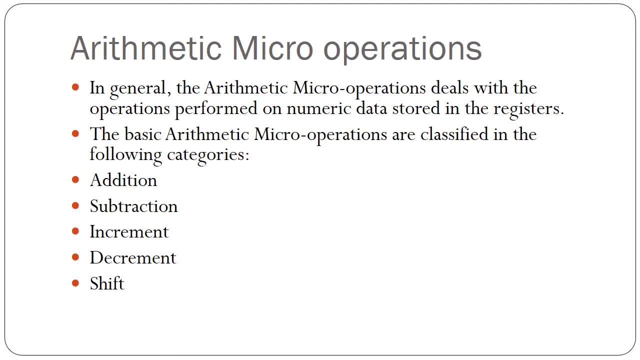 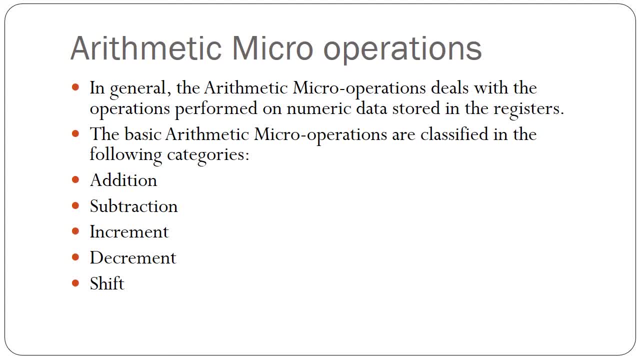 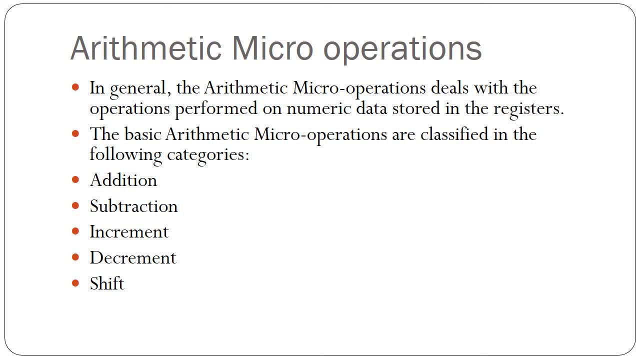 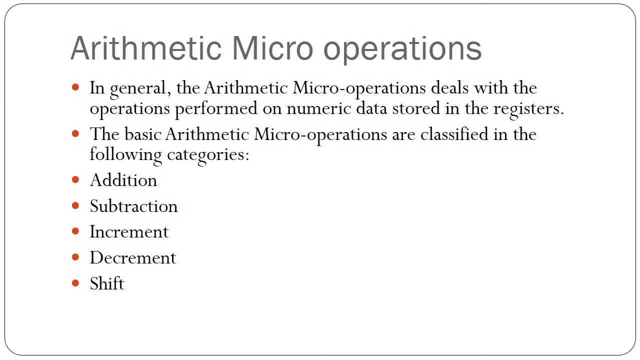 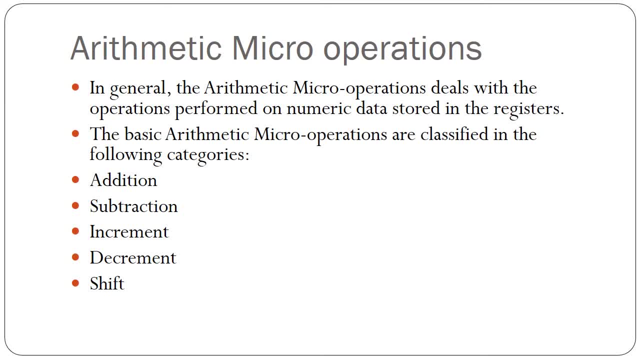 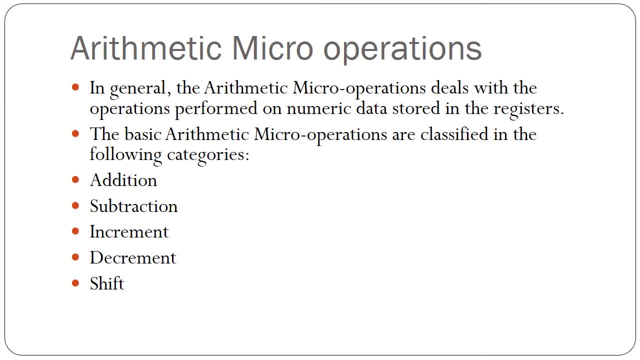